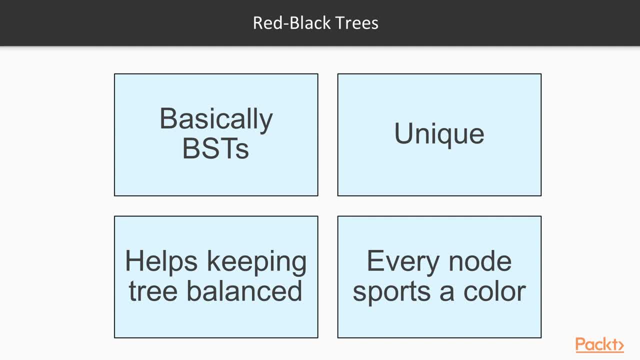 Red, black trees are basically BSTs. However, these trees are unique. Every node sports a color, either red or black. This auxiliary information helps us keep the tree balanced, as we'll soon see. Let's familiarize ourselves with some terms we'll commonly come across. 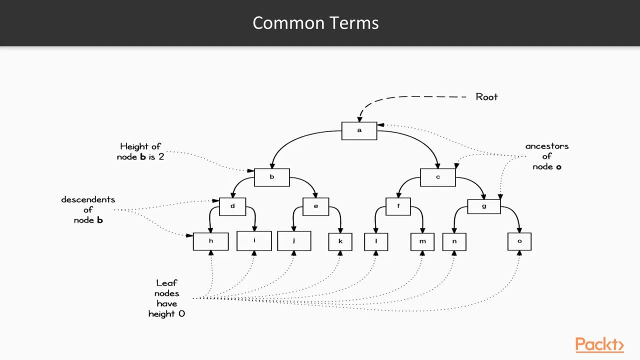 Here's a helpful diagram showing the terms. A tree node's height is defined as the number of edges on the longest path to a leaf. A leaf node's height is 0.. For example, in this diagram, the height of the node H is 0.. 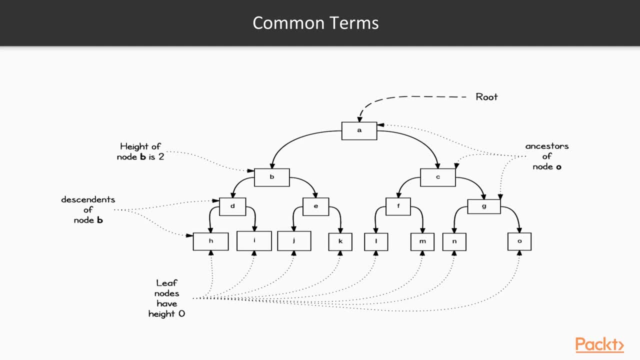 The total number of children of a node is collectively referred to as the node's degree. A leaf node's degree is 0.. Here the degree of node A is 2.. A non-leaf node is also called an internal node. For example, in this diagram, node A is 0.. 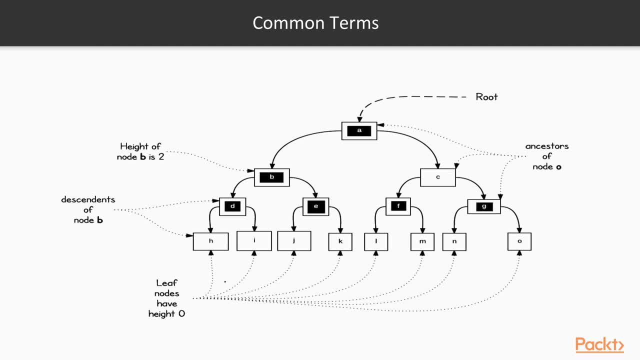 A non-leaf node is also called an internal node. For example, in this diagram, node B is 0.. And node C is an internal node. So are A, B, D, E, F and G. Every internal node in the previous tree has the same degree 2.. This makes the tree a complete binary tree. 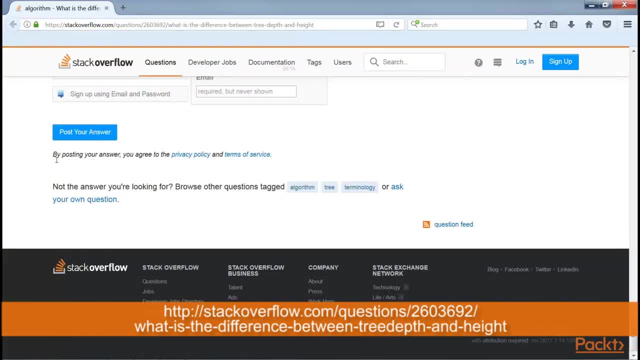 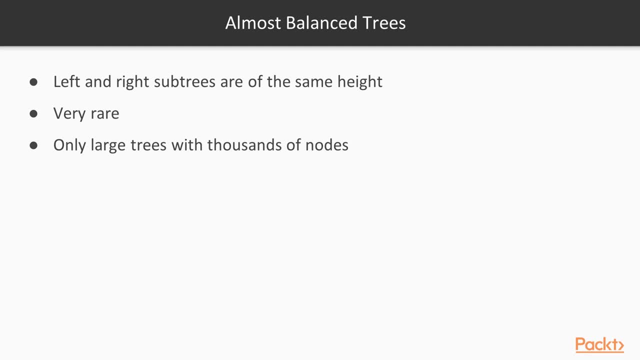 You can refer to this website for more details and related discussion. In the tree we just saw, every node's left and right subtrees are of the same height. This makes it a tree that is perfectly height balanced. However, such trees are very rare. 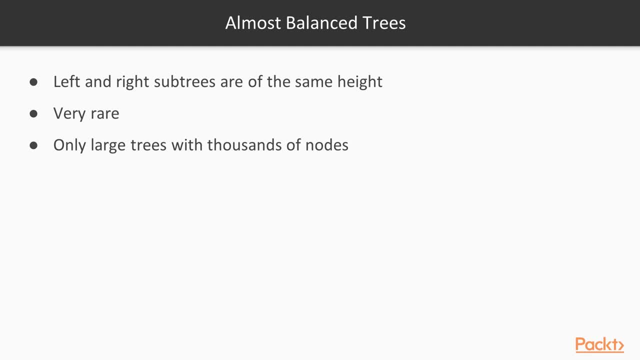 We come across them only when we have large trees with thick branches. We come across them only when we have large trees with thick branches. Instead, we could try for trees that are either perfectly height, balanced or somewhere close to that. Instead, we could try for trees that are either perfectly height, balanced or somewhere close to that. 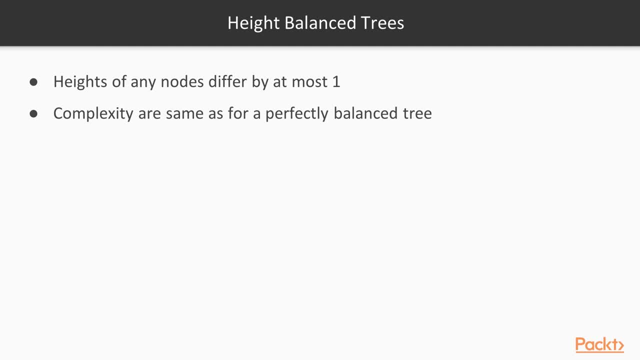 What do we mean by height balanced? If the heights of any nodes differ by at most 1,, it's a height balanced tree. The complexities of various operations would almost be the same as for a perfectly balanced tree. In this diagram, the left tree is height balanced, whereas the right tree is not. 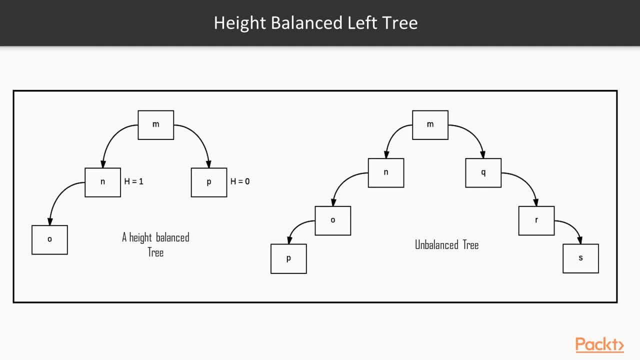 In the left tree, the height of the subtrees rooted at n is 1.. The height of the subtrees rooted at p is 0.. These differ by 1, but we're okay with this little bit of imbalance. Before we jump headlong into the nitty-gritty of red-black tree implementation, let's look at a fundamental concept.